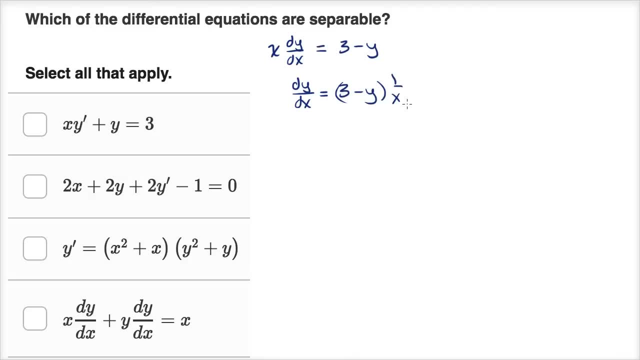 And so it's clear. I'm able to write the derivative as the product of a function of y and a function of x. So this, indeed, is separable, And I could show you. I can multiply both sides by dx, and I can divide both sides by three minus y. now, 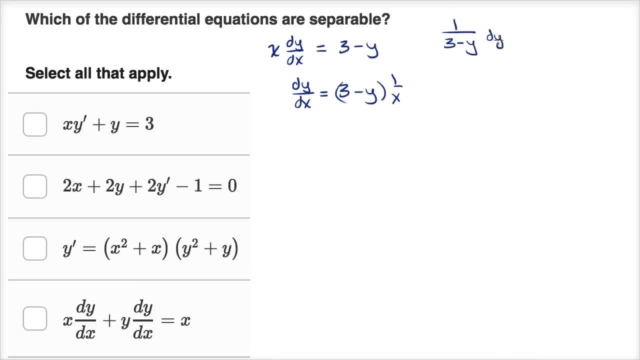 And I would get one over three minus y dy is equal to one over x dx, So clearly this one right over here is separable. Now let's do the second one, And I'm gonna just do the same technique. I'll do it in a different color. 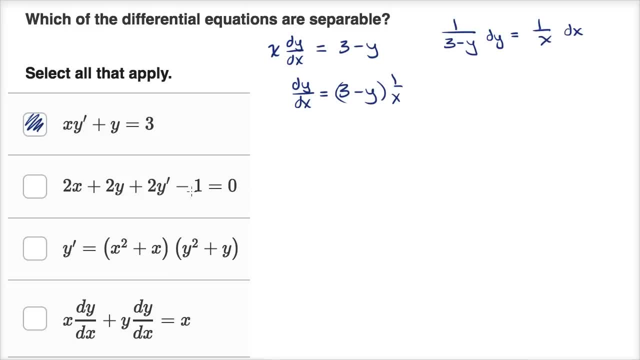 so we don't get all of our math all jumbled together. So in this second one, let's see if I subtract the two x, the two y from both sides. so actually let me just do whoops, let me do a couple things at once. 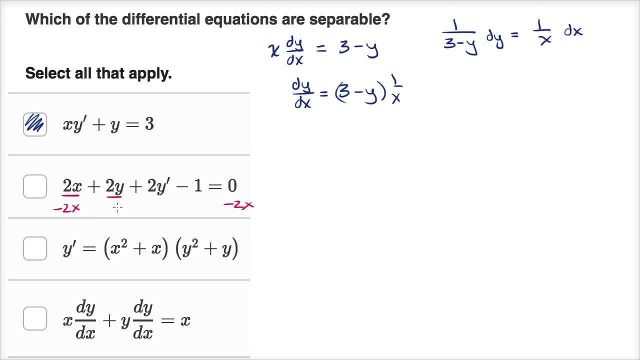 I'm gonna subtract two x from both sides. I am going to subtract two y from both sides. So I'm gonna subtract two y from both sides. I'm gonna add one to oh to both sides. so I'm gonna add one to both sides. 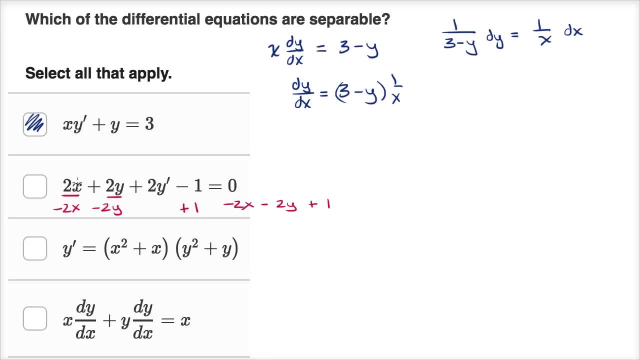 And then what am I going to get if I do that? This is gonna be zero. this is gonna be zero. this is gonna be zero. I'm gonna have two times. the derivative of y with respect to x is equal to negative two x. 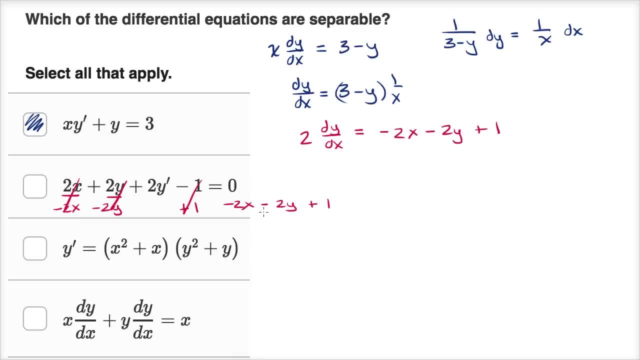 minus two, y plus one. And now let's see, I can divide everything by two. I would get. the derivative of y with respect to x is equal to and actually, yeah, I would get. I'm just gonna divide by two. 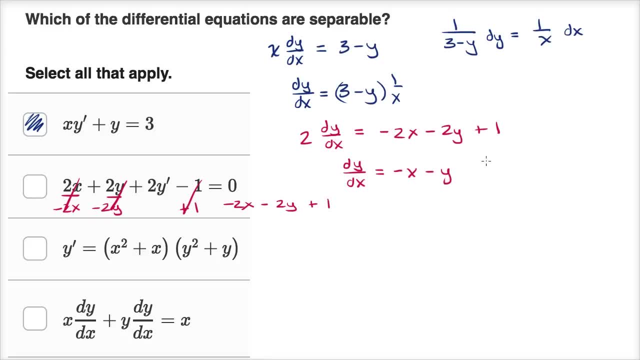 so I'm gonna get negative x minus y, and then I'm going to get plus 1 1⁄2.. So it's not obvious to me how I can write this as a product of a function of x and a function of y. 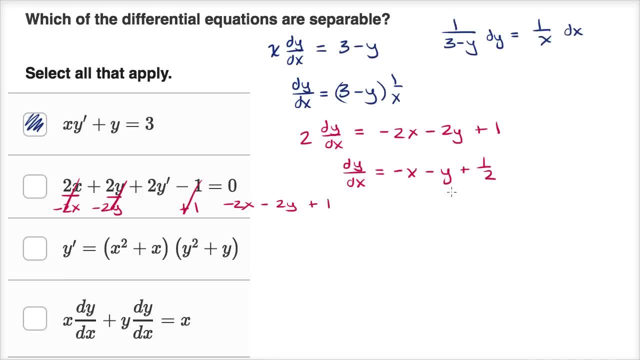 So this one does not feel. this one right over here, is not separable. I don't know how to, how to write this- as a function of x times a function of y. So this one, I'm not gonna I'm gonna say is not separable.